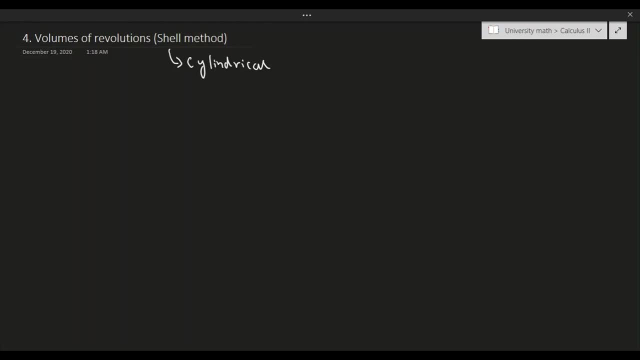 work and how is this different from the method of rings or disk method? So let's go ahead and discuss this with a kind of a conceptual example and as to why this is necessary. So let's go ahead and do this And let's kind of talk about this situation for a second. So here's the example. 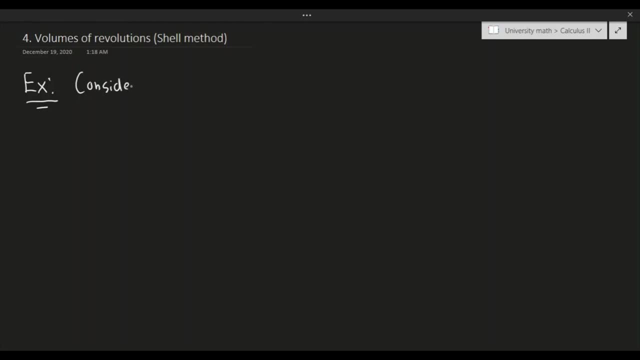 So consider y is equal to x minus 1 times x minus 3 all squared. Here we are going to find the volume. Find a volume by revolving this region, So region about the y axis. So this might seem a little bit out of the blue as to why I'm doing examples for right away, But I promise this will kind of lead. 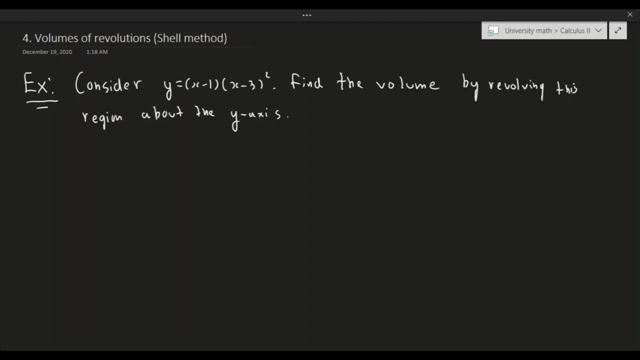 into the idea of this. So let's go ahead and do this. So let's go ahead and do this, So let's go ahead and do this. So let's kind of just talk about this for a second, So to give you a sense. 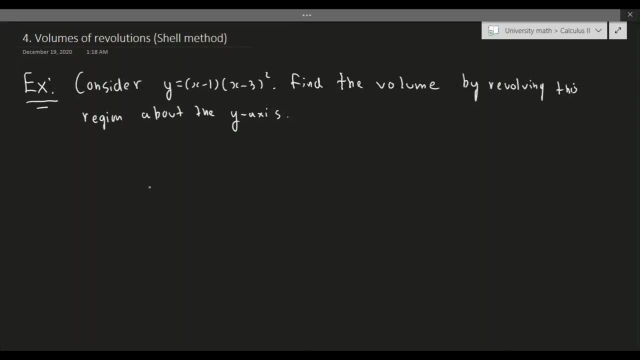 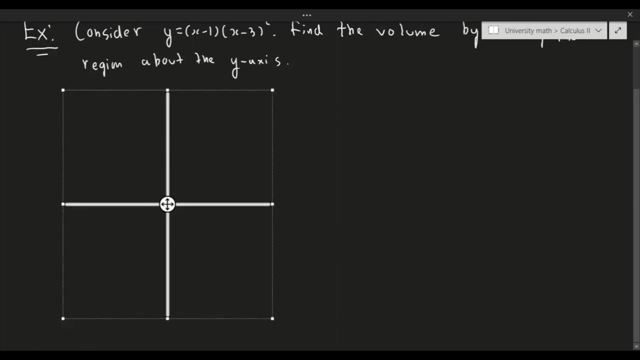 of what this curve looks like. let's go ahead and draw an axis. So here's an axis, And let's kind of expand this a little bit. There we go, Okay, so the graph looks something like this, roughly Or less. Let's just make this a bit neater, So something like this, And then let's. 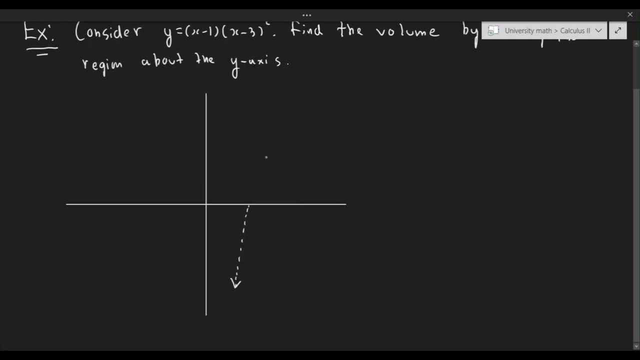 something like that. Okay, so this is one and that's three. Okay, cool, Now let's go ahead. So this is the y axis and this is the x axis. Now let's revolve this around the y axis, So we're revolving it in this direction. Okay, so if we go ahead and revolve, 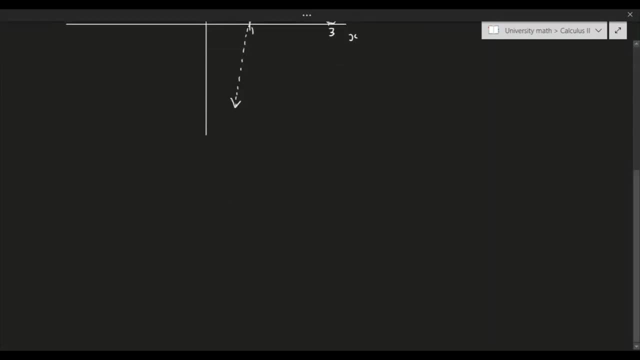 this. that's going to make our situation look something like this: So let's put this here, Let's make this a little bit bigger And let's put this here. There we go, Okay. so if I just look at the actual curve itself, well, that's going to look something like: 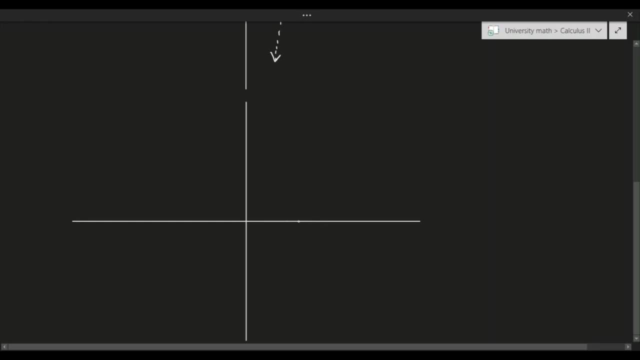 this, something like this, and then something like that. That's for the right hand side. So if I revolve it, it's going to flip around. it's going to look something like this, so to speak. So now, if I made a ring, it's going to look something like this: 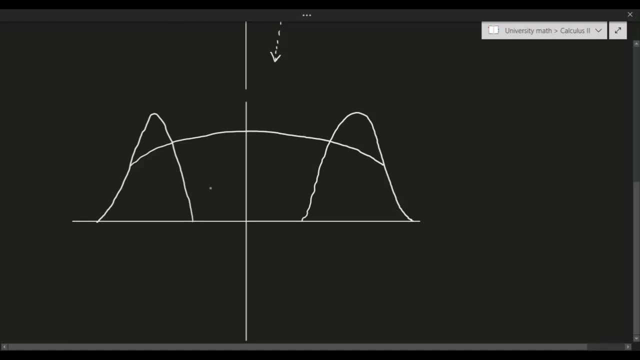 So here's the outer ring And here's the inner ring. that's going to look something like that, But there's several problems here, So let's talk about what's actually going on here. So let's talk about what's actually going on here. So let's talk about what's. 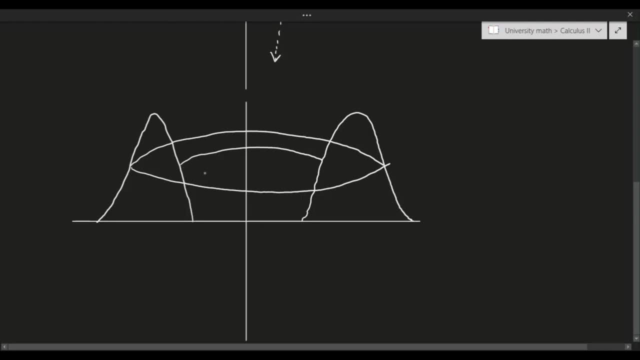 actually going on here. So let's just kind of make this a bit nicer. So that's minus 1, minus 3, and that's 1 to 3, and that's x and that's y. Okay, so let's talk about. 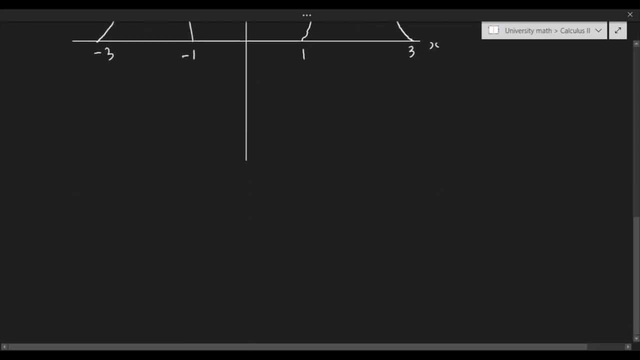 what's actually going on here? The ring is perpendicular to the y-axis. We can clearly see that it's perpendicular to the y-axis, So the equation that we need for the rings have to be in terms of y. So let's kind of talk about this. So y- we're going to talk about this. So y- we're going to talk about this. 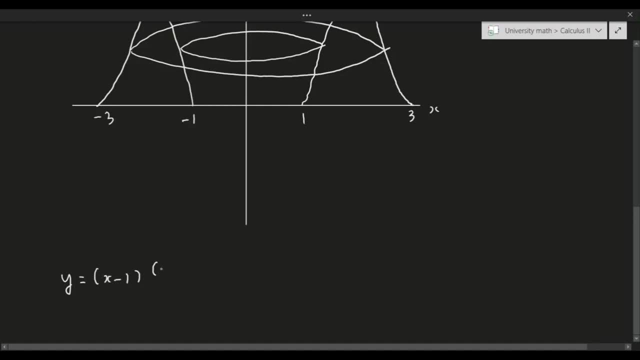 is equal to x minus 1 times x minus 3, all squared. The ring has to be perpendicular to the y-axis. So the problem is that because it's perpendicular to the y-axis, we have to solve this equation for x. So solve for x. Unfortunately, that's really difficult, because this, if I were, 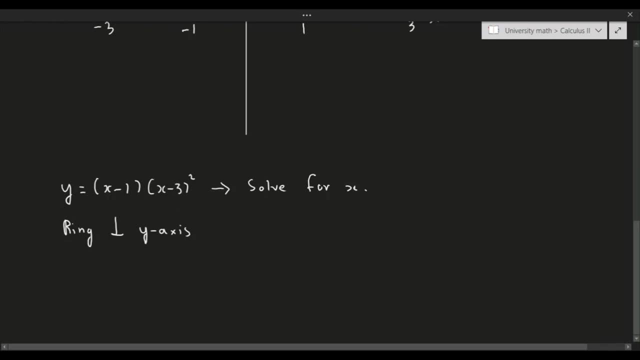 to expand this function out. this would be a cubic equation, And solving a cubic in general is almost always impossible, if not at least very difficult. So generally, solving a cubic is just it's not the best thing to do, So bad idea. So this isn't really possible in this situation. So what can we do? We can't really use. 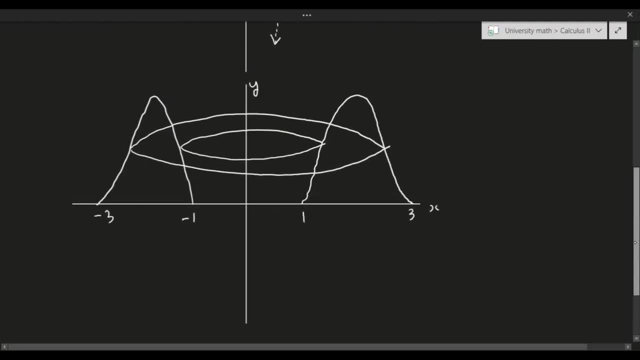 the method of rings here, because, number one, the height will vary as a function of y as we go up or down this graph. So that's going to be even harder to deal with. And number two, we would have to solve for x anyway, And that's just. 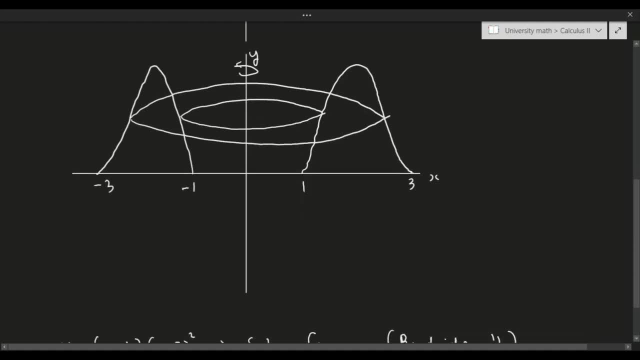 really difficult. So is there another way we can kind of solve this volume of revolution? Yeah, we can actually use something called the shell method. So earlier all our cross sections were either rings or disks in some way, But that doesn't necessarily all have to be the only cross. 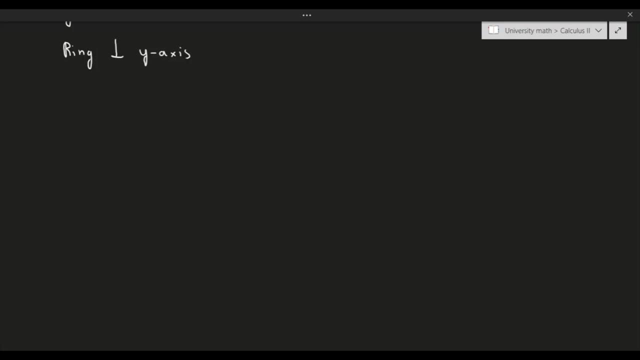 section. If you recall the first video, when we did about volumes of revolution, some of our cross sections were rectangles, some of our cross sections were disks and so on. In the case of the pyramid, it's a square bow, square cross section, So it doesn't necessarily always need to be a ring or a disk. 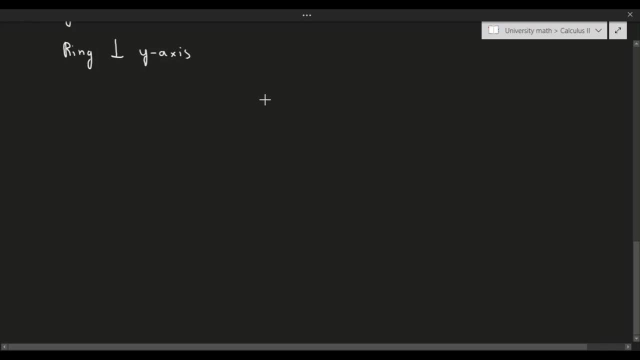 We can have, we're allowed to have other cross sections. So how do we deal with this situation? So let's go ahead and draw an appropriate cross section. that lets us kind of deal with this a lot easier. So, once again, here's the graph. Here is another part of the graph. Let's go ahead and draw a. 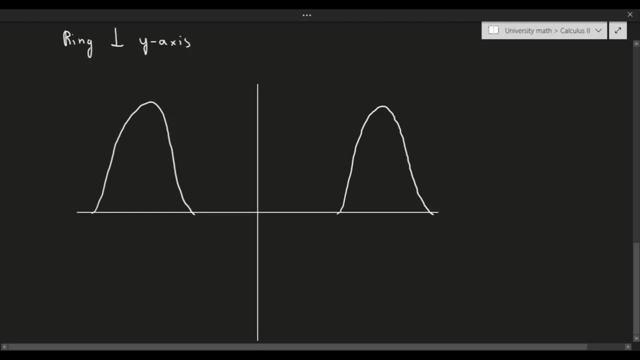 cross section. That's kind of nice. So what kind of cross section can we use? Well, one thing we can do is we can pick a cylinder to be a cross section. So how does that work? Well, here is the top half of the. 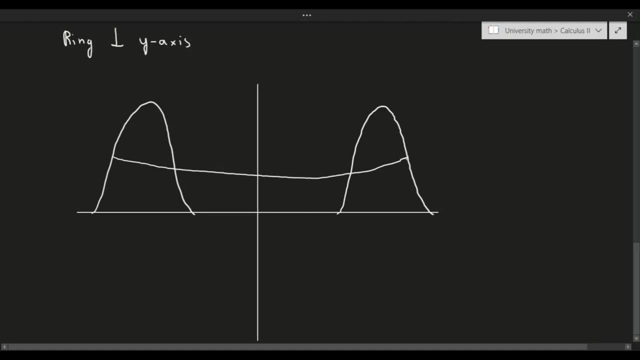 cylinder right here. And here is the cylinder going down. And this, right there, is the base of the cylinder, And here is the other part of the cylinder. Okay, so why is this different from the method of rings And how is this more helpful? Well, here, the nice thing is that the radius is going to be distance, since we're 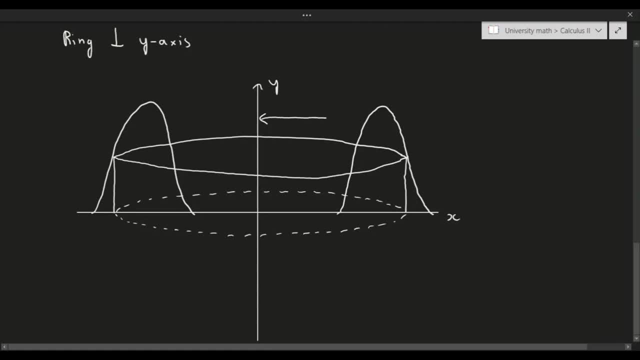 revolving this around the y axis, So like. so the radius is going to be the distance from the y axis to some distance, x on the graph. So, since we want a full radius, that would be this entire distance. So, as a result, we're going to have a distance of x. So we're going to have a distance of x. So we're going to have a. 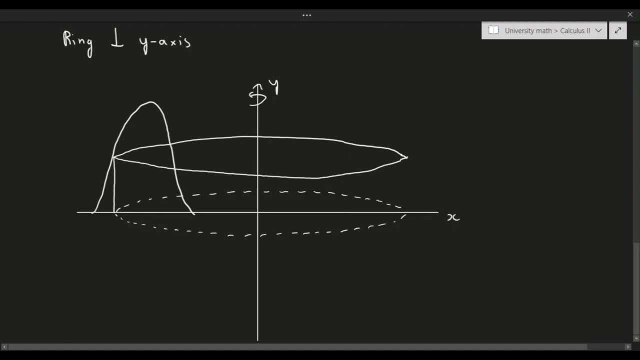 The result. let me just use a different color to do this. I'm going to do that, Okay. so if I went, if I go ahead and draw a use a different color to this. as soon as there was that arrow, There we go. Okay, so we just redraw that part of the. 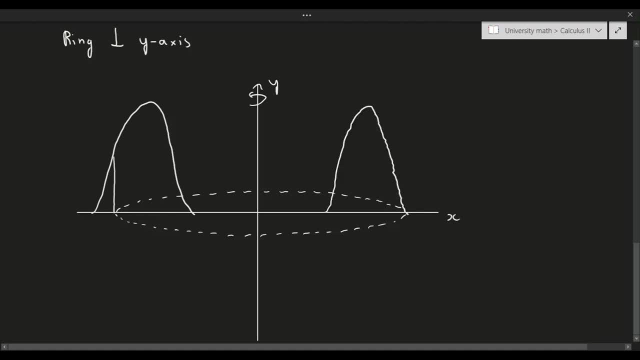 graph. Okay, so let me just go ahead and draw the cylinder again. There we go, alright, Okay, so let's just finish that part off And there. Okay so now the distance. so let's use a different color to do this. 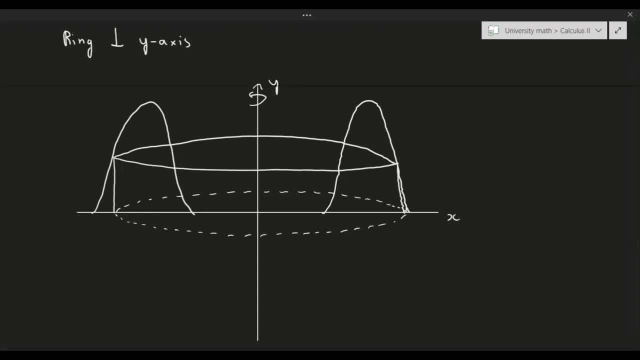 So let's use green. So the distance between the y-axis and the end of this graph would be the radius of the cylinder. So this right, there would be the radius And this distance. we'll just call it x, because the distance from the y-axis to any point. 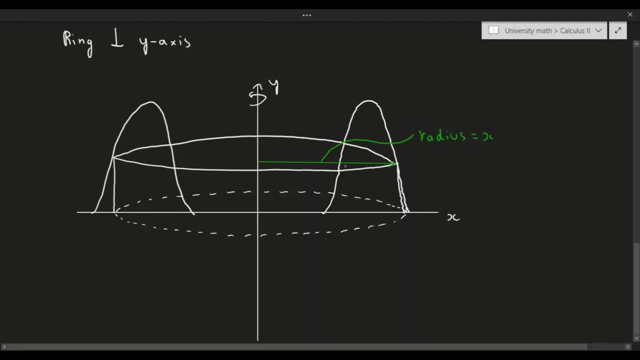 any point on this graph will be some x- distance. Now what's the height? Well, the nice thing here is that the height is much easier to measure. The height is just going to be some distance y. So this would be the height. 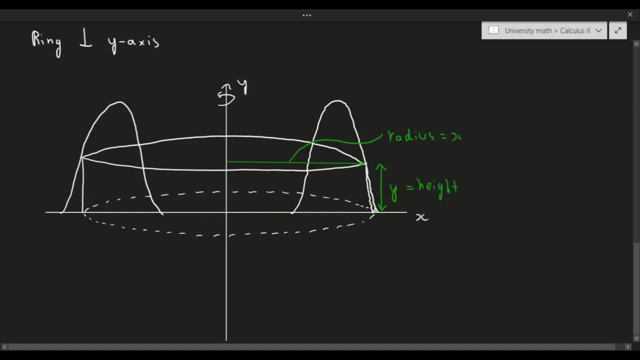 Okay, And the nice thing is because the y is defined in terms of x explicitly, it doesn't matter where we are in the graph. If we made our cross-sections here, for example, the height would be whatever distance it is. 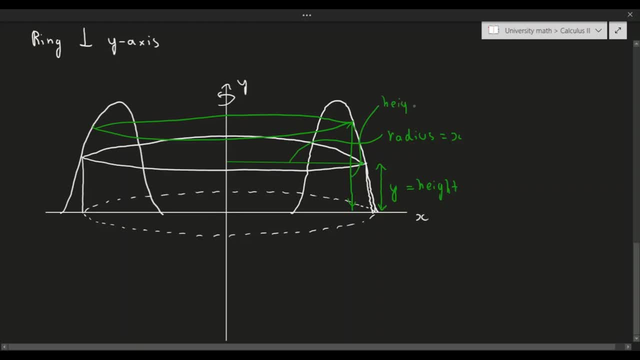 So this, in this case, this would be the height, And that would also be equal to y, And the radius, and, as we can see, the radius is still going to be the distance from the start of this y-axis to the end of this axis. 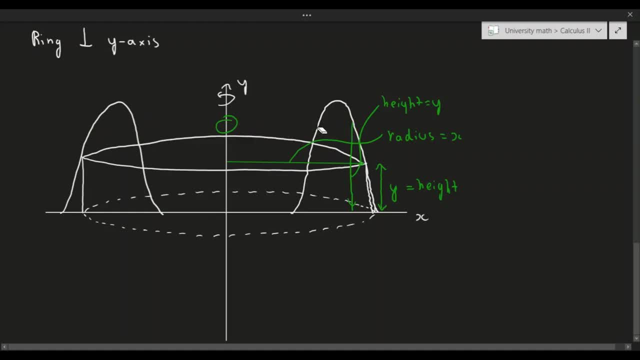 So it doesn't really matter where you pick your cross-sections to be Okay, As long as the cylinder starts at some point, we can go ahead and define some distance. It doesn't really matter. So the height is going to be some distance. y and the radius is going to be some distance. 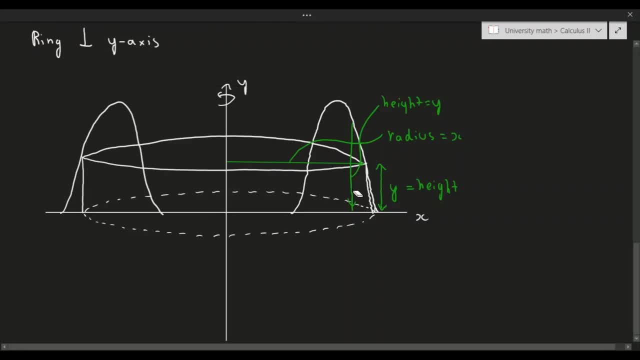 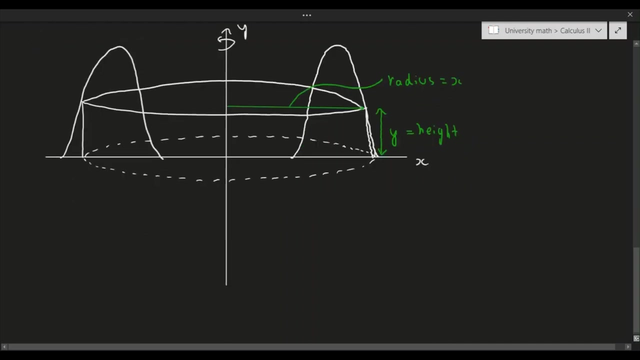 x. And the nice thing is that, because our height is defined in terms of y explicitly, we can go ahead and define this in terms of x only. So that's very, very nice. So let's go ahead and kind of talk about how to actually do this. 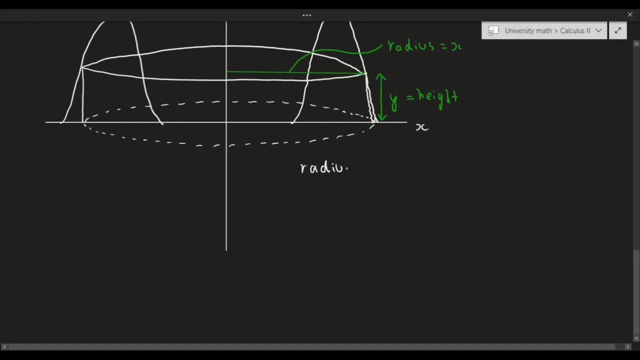 So just to be very clear, the radius is equal to x and the height is equal to y, So the surface area, or one kind of small slice of the cylinder. so if I were to look at a really small slice, for example, the surface area of the cylinder would be 2 pi. 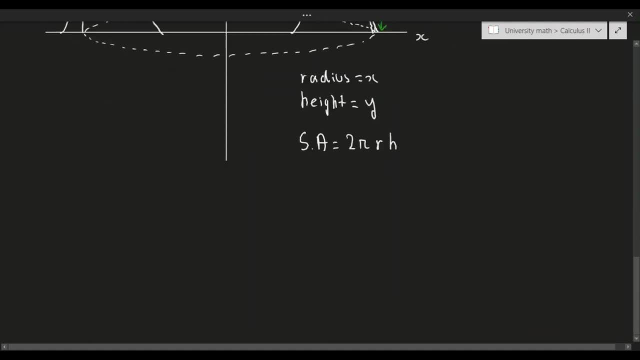 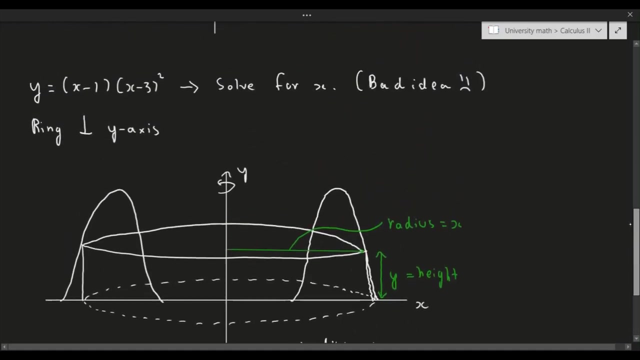 times the radius, times the height. Okay, So now we know the radius, in this situation, is just going to be x and the height, well, it's just going to be y. But we know what y is equal to. According to the question, y is equal to x minus 1 times x minus 3, all squared. 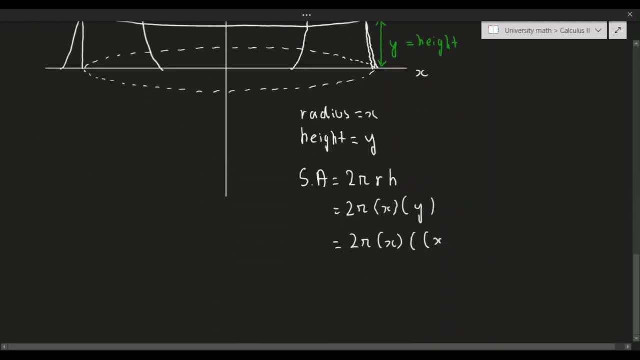 So if we go ahead and write that down, we'll get x minus 1 times x minus 3 all squared. Okay, So in this situation the volume would be x minus 1 times x minus 3 all squared. Okay, So in this situation, the volume would be x minus 1 times x minus 3 all squared. 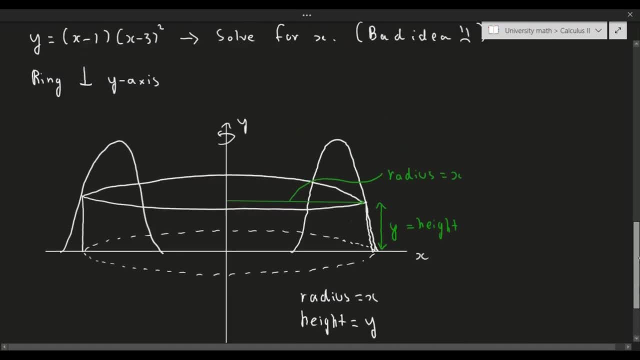 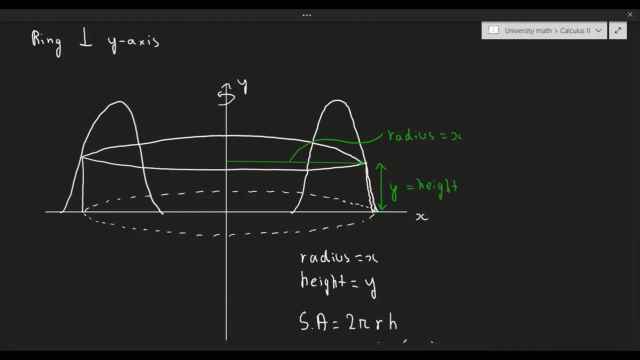 If you see the integral of these small kind of disc-like surface, of these discs-like cylinders, integrated over its distance. So what do I mean by that? Well, this kind of point, right, there is 1, and that's 3.. 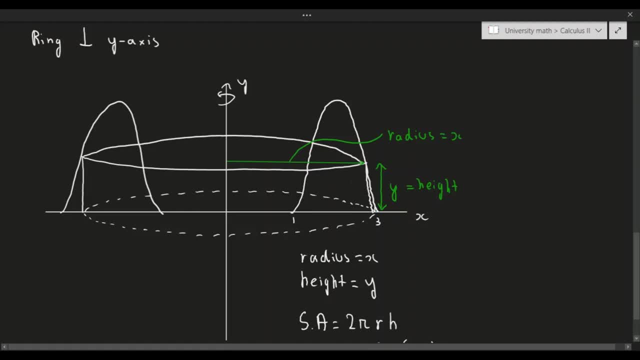 So what we're gonna be doing is integrating all these little cylinders from 1 all the way to 3.. If you can do that, we would have covered this entire kind of volume as a result. Okay, us our total kind of volume for this volume of revolution. So just to be very clear as to what's. 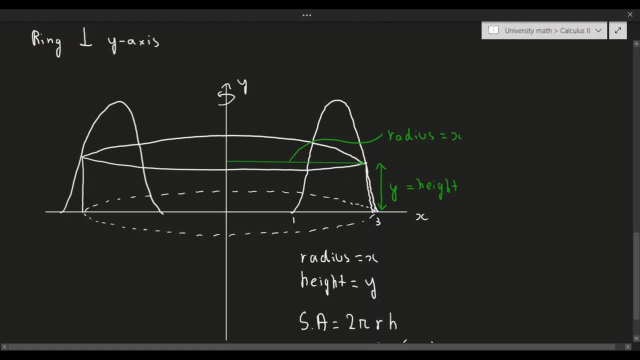 going on here if you start at one. so just to be very clear, let's use blue to kind of illustrate this- If you start at one, we get this small kind of cylinder right there. I'm going to use a circle for reference, but it is a cylinder, So it's going to look something like that. So actually, 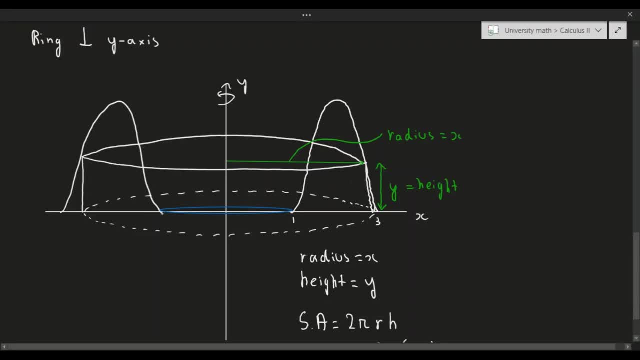 I'm just going to go ahead and do the whole thing. So the cylinder is going to look something like that, for example: at x equals one. At x equals two, it's going to be a bit bigger. At x equals three, it's going to be a bit more. X equals four, it's going to be a little bit more. 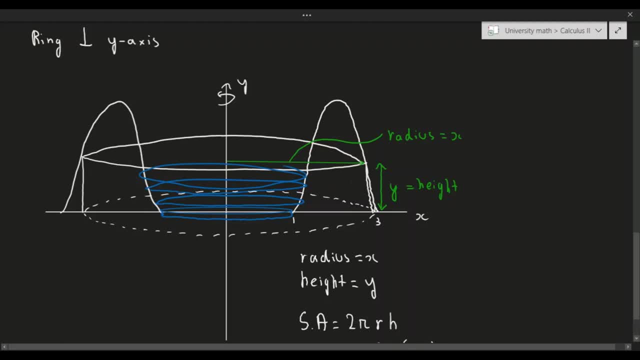 X equals five, and so on and so on. So I made a bit of a jump there, But my point is that at x equals one, the distance between the volume that we're calculating is essentially just going to be this entire distance, right there. 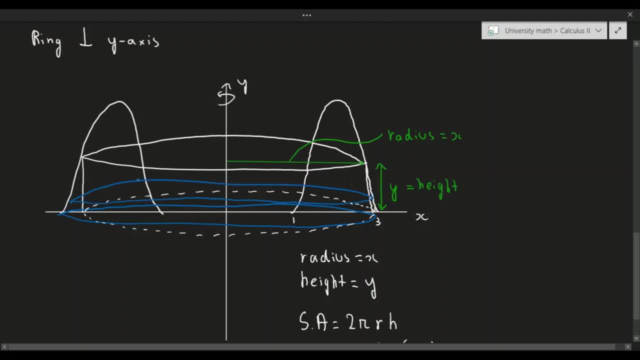 At x equals two, it's going to be this: one At x equals 2.5, it's going to be this: distance At x equals 2.6, it's going to be this. distance At x equals 2.7, so on and so on. So the point is that 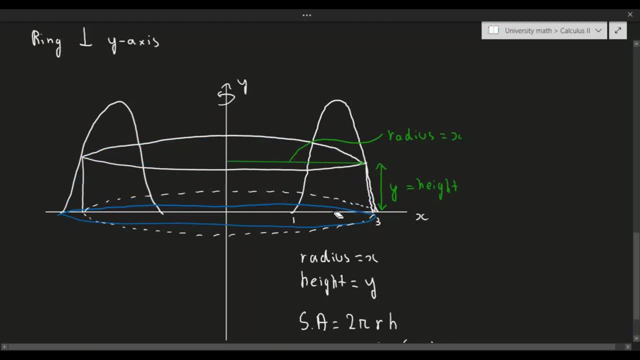 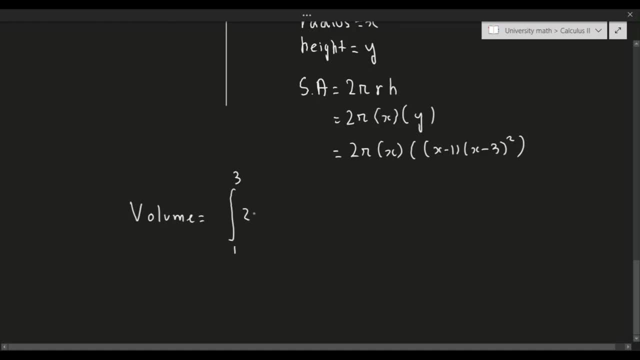 from 1 to 3 of 2 pi times x times x minus 1, times x minus 3, all squared times dx. Okay, we can take the 2 pi out, so we get 2 pi times the integral from 1 to 3. 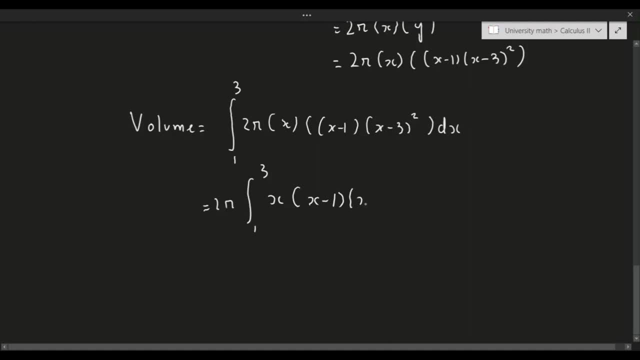 of x times x minus 1 times x minus 3, all squared times dx. If we expand this out, we'll get x to the 4 minus 7x cubed plus 15x squared minus 9x times dx. Okay, so if we integrate this, we'll get 1 over 5x to the 5 minus 7 over 4 x to the 4. 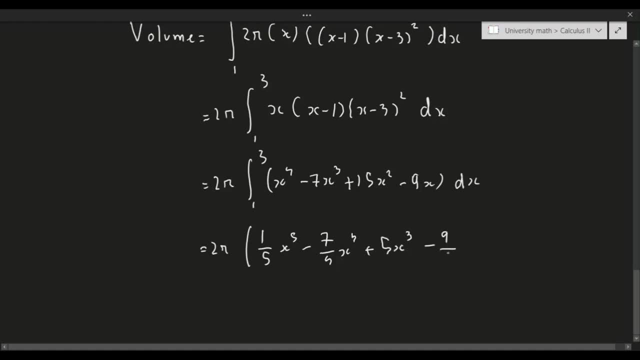 plus 5x cubed, minus 9 over 2x squared, and then we integrate that from 1 to 3, and if we do that we'll get 24 pi over 5. so that would be our final answer. so let's kind of recap. 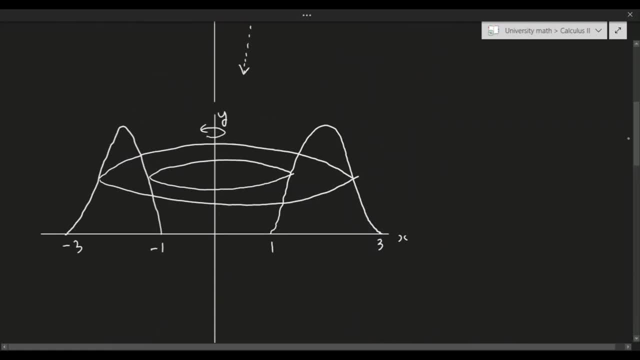 what we did here. using disk method would be a little bit harder than it normally would be that you'd be used to, just because of the fact that in order to use a disk method, we have to solve this equation for x, and generally that's not really that's not very easy. 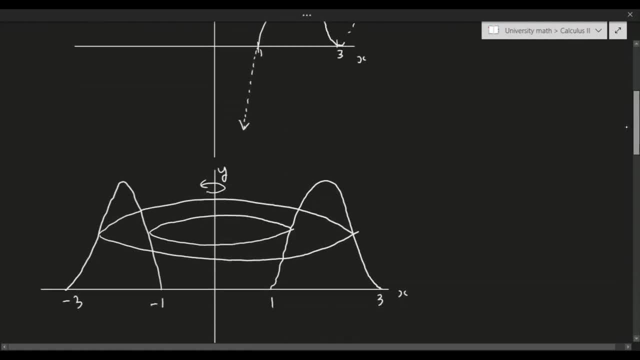 for a cubic equation such as this one, and the reason is because the, the disks here, or the rings, are perpendicular to the y-axis. so, as a result, we have to make sure that the equation that we use is actually in terms of x only, or rather in terms of y. so we have to take 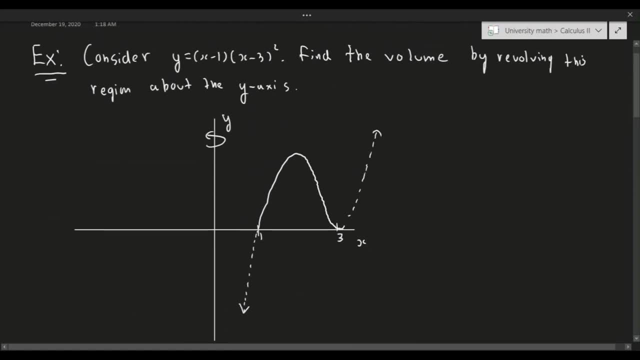 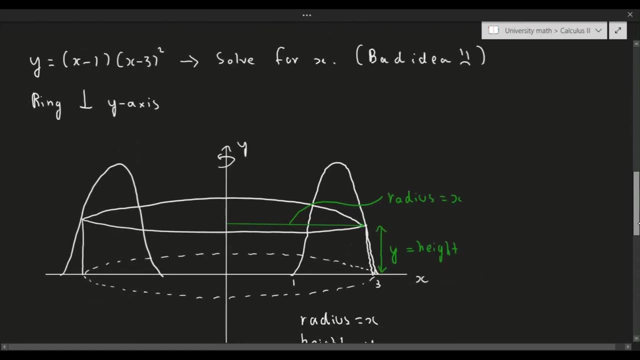 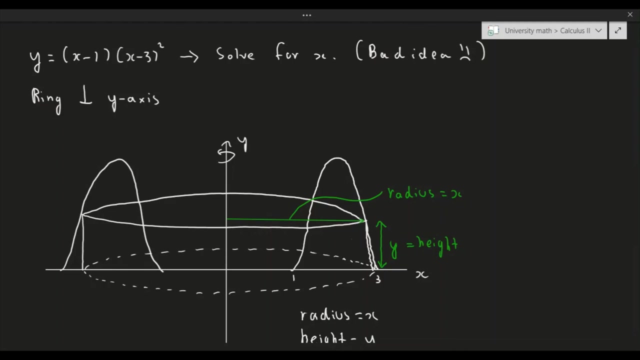 the equation that we were given right here and solve for x. so that's not very easy to do for a cubic, so this isn't quite going to work. so instead we use a different cross-section, which would be a cylinder this time. the cylinder is much easier to work with, because as soon as we kind of increase the heights of the cylinder, as soon 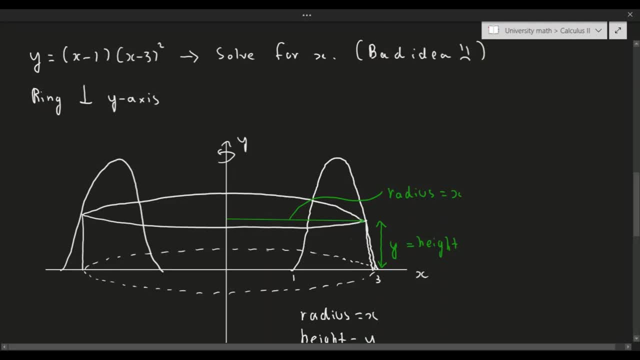 as we start with 1, at x equals 1, we get this cylinder. at x equals 1.5, we get this cylinder. at x equals 1.75, we get this cylinder, and so on and so on, so as we kind of go from 1 to 3 using 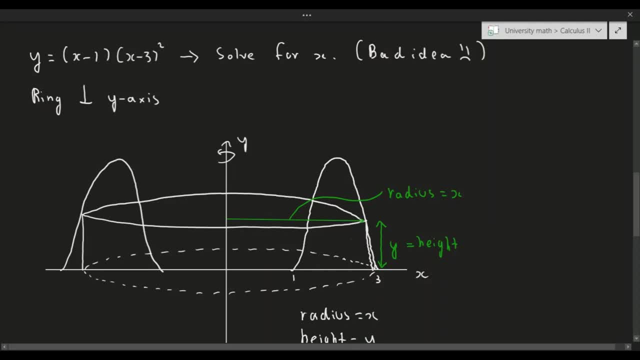 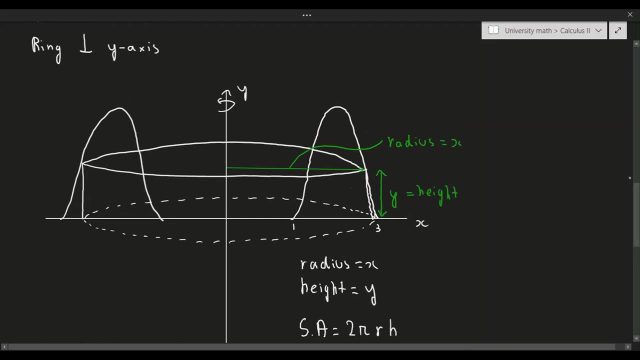 a cylindrical cross-section. we go from the bottom of this graph to the top of this graph, which will give us our total kind of volume. so the shell method basically works like that. excuse me now, it must be noted that, regardless of which method you use, you will always get the same answer, since the volume of an object will never change regardless. 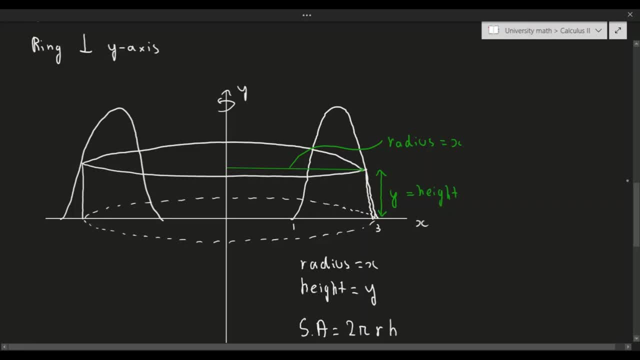 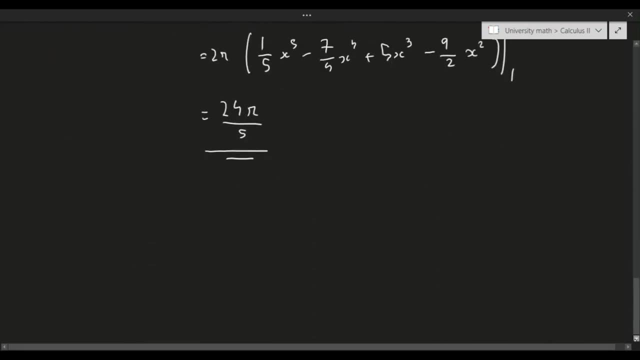 of which better to use. but sometimes it's easier to use one method versus the other, depending on what kind of graph you have. so let's go ahead and do another example of this shell method technique. so let's go ahead and do this example. so find the volume of the solid of the region bounded by. 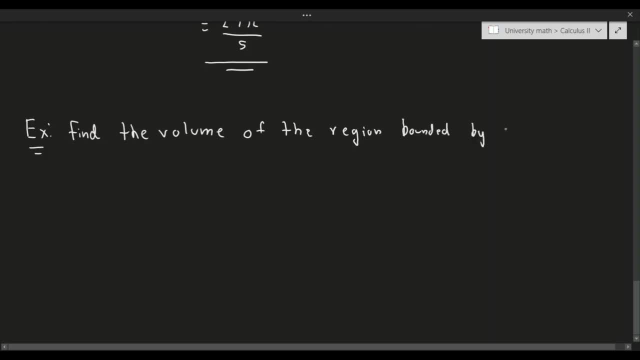 y equals x squared plus 4x. so we're just going to make that bit neater: y equals 0 and x equals 1 and x equals 4. about the y-axis: okay, so let's go ahead and draw the situation out. so here's my axis once again, so it sees from x. 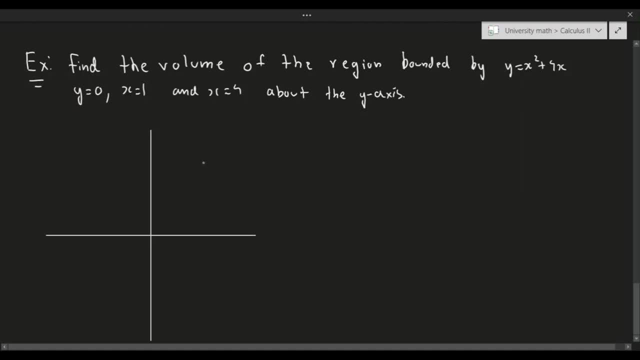 equals 1 to x equals 4. so from that point on, from those points only, the graph is going to look like that. so let me just make this a bit nicer, so something like that. so this point, right there, that's one, that's four. so if I revolve this around the y-axis, so this is y, that's x, that's going to. 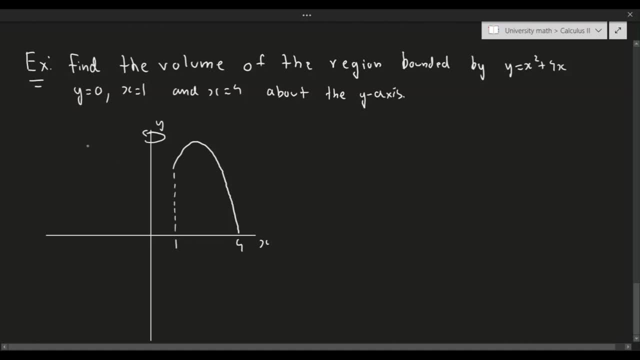 look something like that. okay, so if I go ahead and draw a cylinder once again, so just to be very clear, that's going to look something like that. so if I go ahead and draw a cylinder for this situation, well, that's going to look something like this. 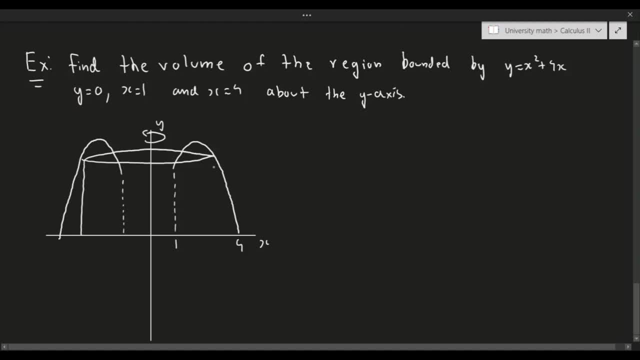 now it is not necessary to necessarily draw the cross-sectional areas, but it can help sometimes in visualizing what's actually going on. so let's go ahead and do that. so this just be very clear. that's one. that's four. so good, I've already done that. 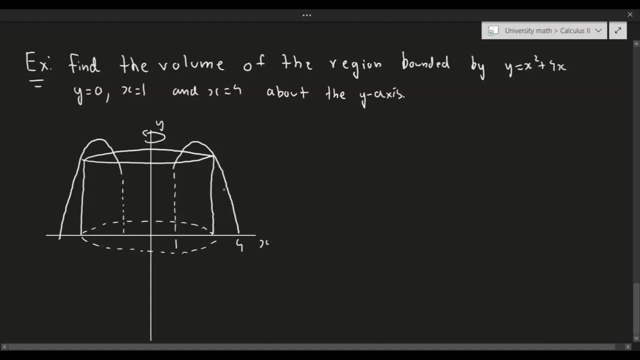 so as a result- well, let's talk about the height- is the height in this situation would just be equal to y, but the y is equal to x squared plus 4x. now what is the radius? so the radius is the distance from the y-axis to the end of the graph. so let's go ahead and 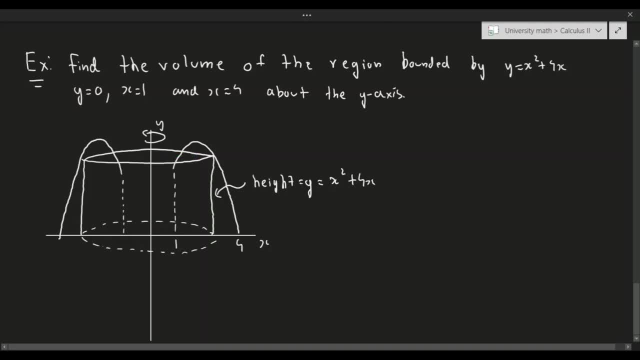 draw that out, so let me just go ahead and erase that, because that was really neat. okay, so this would be the radius, and in this situation the radius is equal to. well, that's just equal to x, because the distance from the y-axis to the end of the graph is the sum distance, x. it will change depending on where I 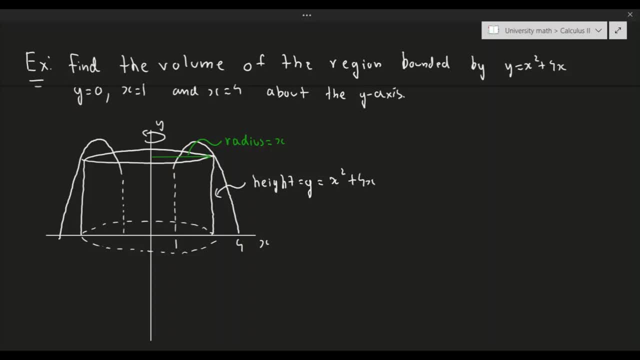 am on the graph. so, for example, right here, if I would draw my cross-sections right here, notice the distance would still be to the end of the graph, so the distance would still just be x. it's not going to change or something. it's fixed. so let's go ahead and calculate the surface area. 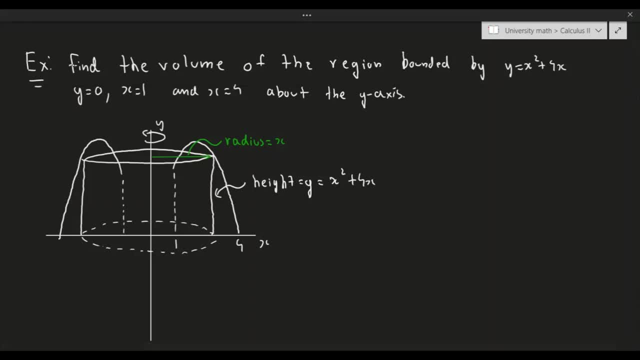 so the surface area. so we just go back to white on this one. so the surface area in this situation is equal to 2 pi times the radius times the height. so it's 2 pi times the radius, but the radius is just equal to x times the height, but the height is just equal to. 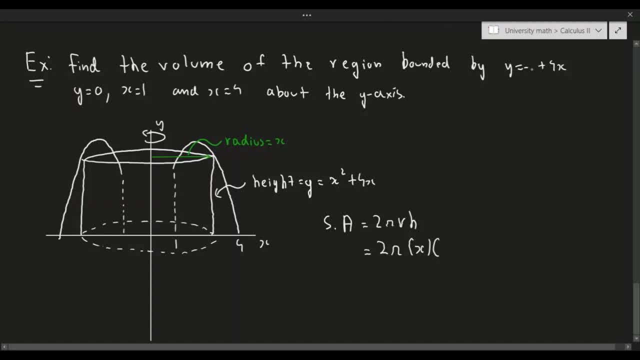 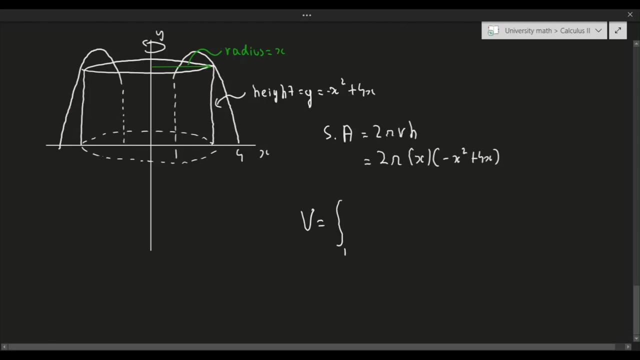 so let me just go ahead and do that. oh sorry, I should say minus x squared, and that's going to be minus x squared plus 4x. so that's going to be minus x squared plus 4x. so let's go ahead and integrate this. so the volume is going to be the integral from one to four of two pi times the. 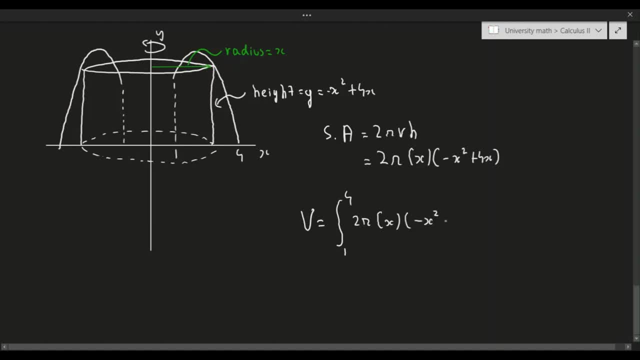 radius times the height, so x times minus x squared, plus 4x times dx. okay, so if you go ahead and integrate this, we'll get 2 pi times. so if I kind of explore this out and do some simplifications, we'll get minus x to the 4 over 4, plus 4x cubed over 3, and then we're going to integrate this. 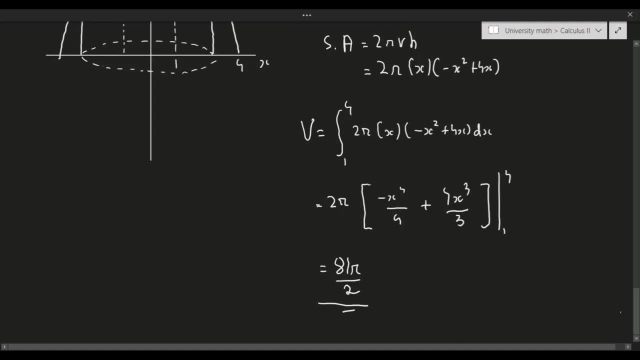 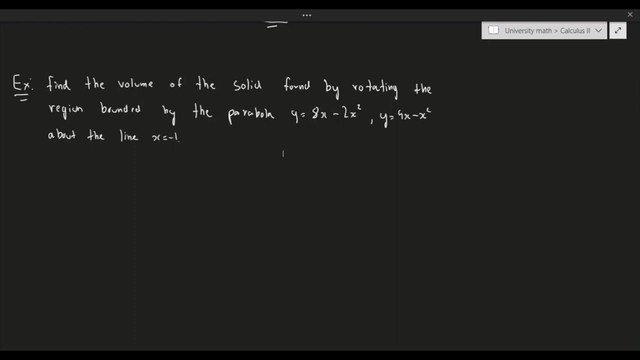 as our final answer. okay, so that takes our bad example. so we have two more to cover. so let's go ahead and talk about how this works. so let's talk about this example. okay, so for this, for this example, let's say: find the volume of the solid found by rotating the. 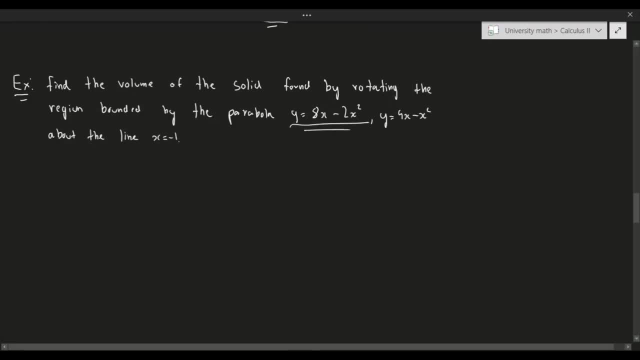 region bounded by the parabola, y equals 8x minus 2x. squared, y equals 4x minus x. squared about the line x equals negative one. so this time we're not rotating about the y-axis. we actually rotate, or the x-axis for that matter. we're. 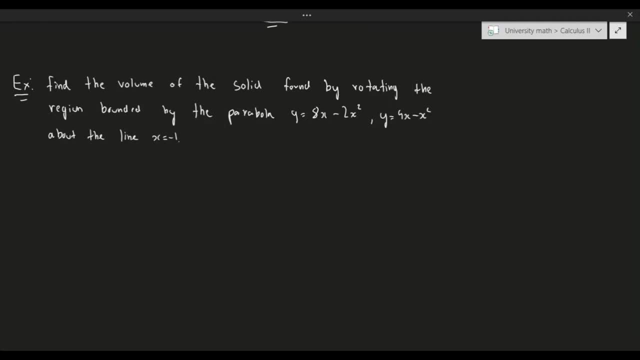 actually rotating this about a specific line. so before we do anything, we should probably find the intersection points for this, for these graphs, because we need to know, we need to know the region of integration. so let's go ahead and do that. so if we intersect these two curves, we get. 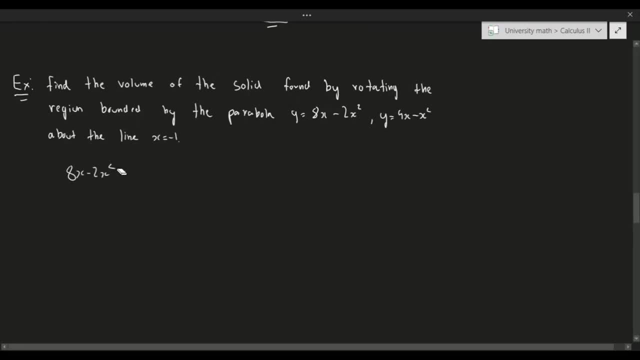 8x minus 2x squared equals 4x minus x squared. so if we move, move everything to one side, we'll get x squared minus 4x is equal to zero. x times x minus 4 is equal to zero. x equals zero and four. so that means our region of integration. 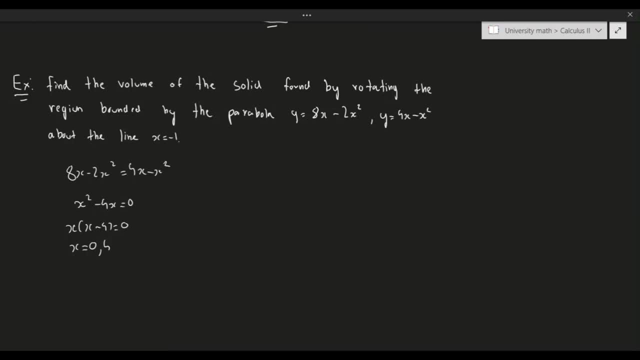 is going to be from zero to four. so now we need to figure out the radius and the height. so we should probably draw a diagram of some kind. so let's go ahead and do that. so add zero the graph, and for the graph is also zero, so our graphs are going to look something like this. so here is the. 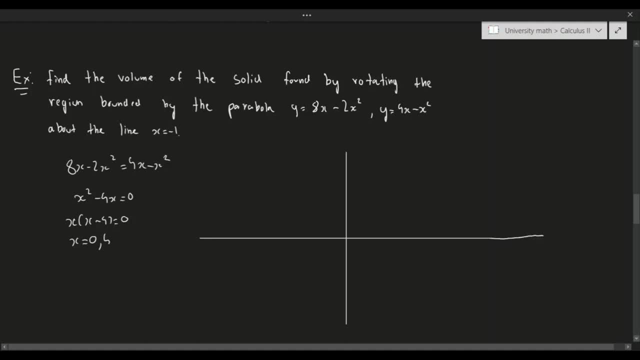 first one. so let me just make this a bit bigger. here's the first one, and here is the second one, so something like that. okay, let me just make this a bit better per se. there we go and there we go, just going to make this a little bit. 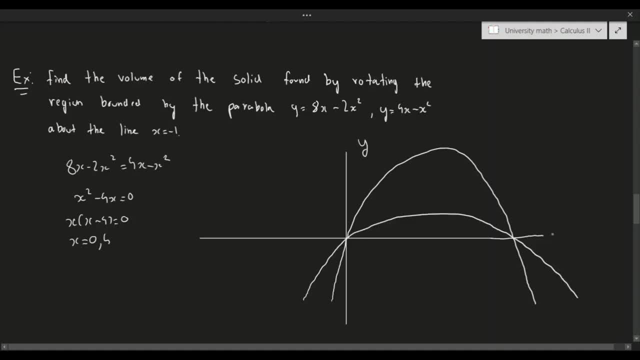 better. okay, there we go. so that's the y-axis and that is the x-axis. so we're going to be revolving not around this line, but the line we will be revolving around. the line x equals 801. so that's about here per se. now this is. 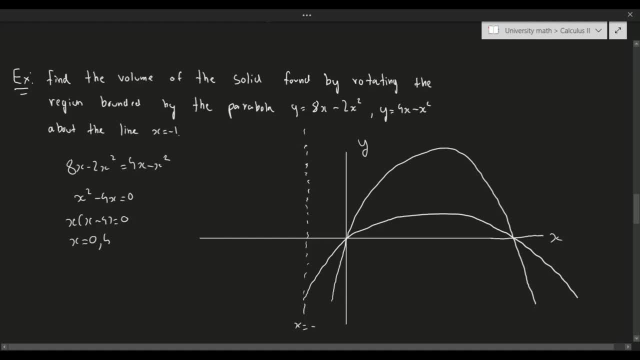 the rough sketch. it doesn't have to be perfect, so x equals negative one. we're going to be revolving around this line, so our next- uh, our region- is going to look something like this: so let's just go ahead and draw an extension of this graph, so something like that. 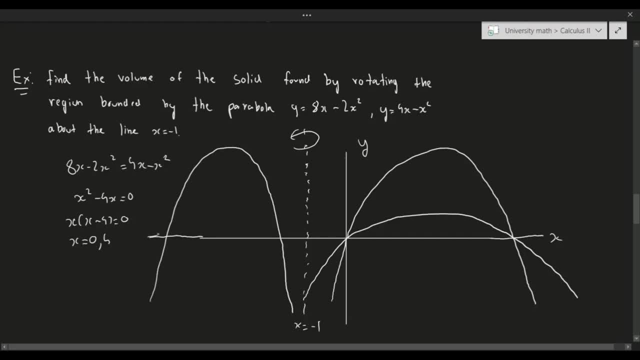 and something like this per se. okay, so our cylindrical region is going to look something like this, so let's go ahead and draw this out. so here's the first cylinder, and there we go, and here's the second kind of base of the cylinder. okay, so that's the cylinder. 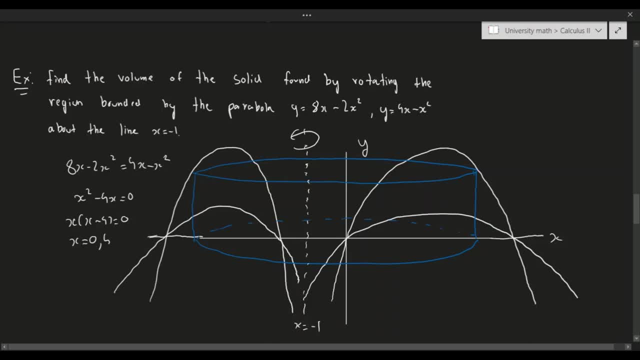 okay, so now the radius of the cylinder. well, that's just going to be x minus minus one. so let's just go ahead and illustrate that using another color. so the radius of the cylinder, that's just going to be this thing. so that's going to be x minus minus one or x plus one. the height of the cylinder is going to be the. 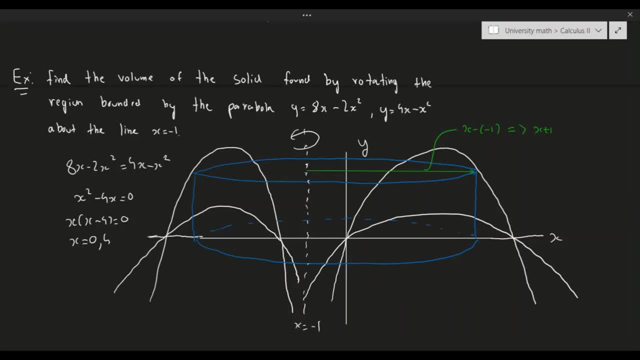 difference between these two curves. so just so, just be very clear before I kind of move on. okay, this parabola right there. so let me just go ahead and write this out: this parabola is 8x minus 2x squared. and this parabola right there is 4x minus x squared. 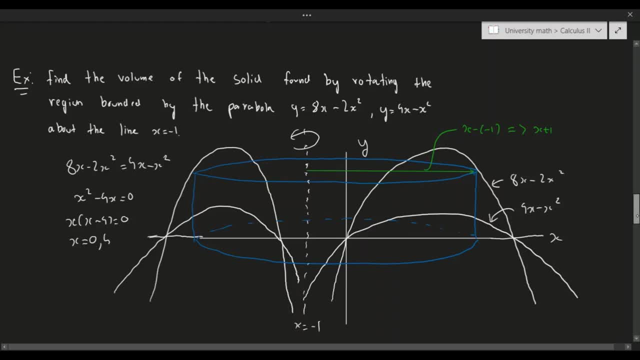 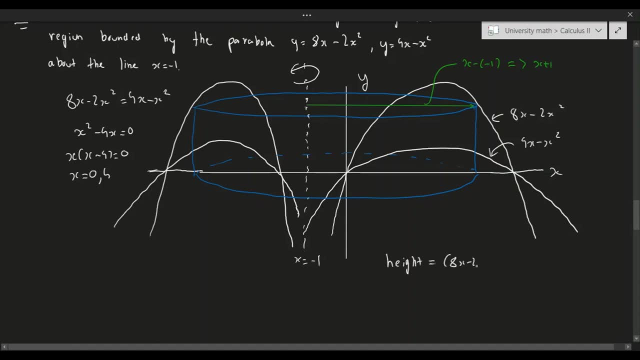 okay, so the height of this, of this kind of figure. so the height is equal to 8x minus 2x squared, minus 4x minus x squared. so if we go ahead and take the difference of these two things, we'll get minus x squared plus 4x. okay, so that means that the height of this kind of figure is going to be. 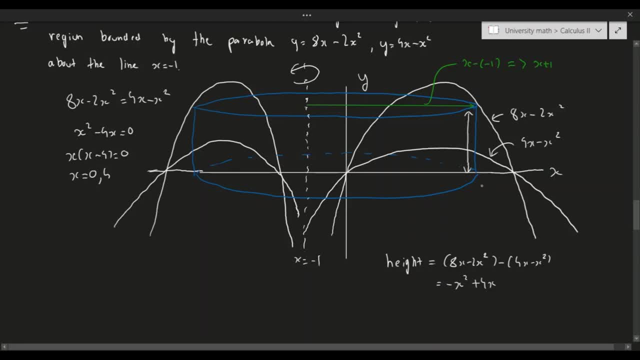 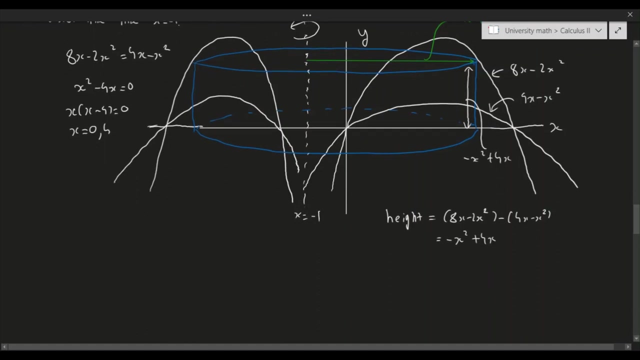 so this height right there, that's going to be this thing right there. so that's going to be minus x squared plus 4x. okay, so that's going to be that particular height. so now we have to go ahead and actually integrate this by integrating the cross-sectional surface area. so we know the bounds and we know. 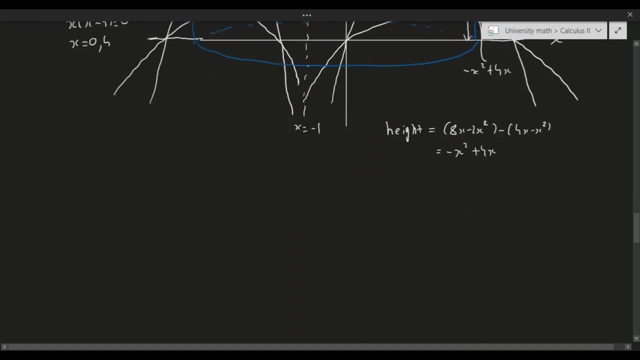 the radius and we know the height. so let's go ahead and do the integral of this. so the surface area is 2 pi times the radius, times the height. so 2 pi times the radius, which is x plus 1, and times the height, which would be the difference. 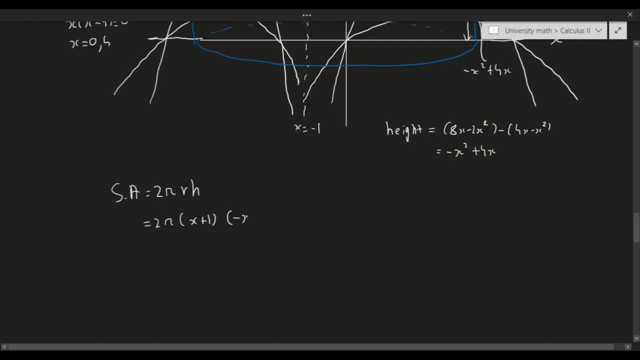 between the two kind of curves. so that's going to be minus x squared plus 4x, which we just found right there. okay, so now we're going to. the volume would be the integral from 0 to 4 of 2 pi times x plus 1 times minus x squared plus 4x times the x, and then we just simply integrate this. 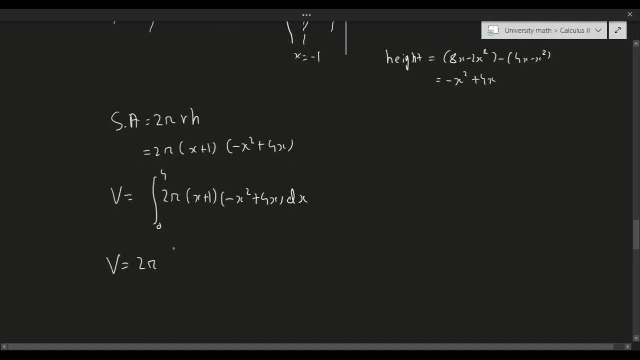 so it's going to be, the volume is 2 pi times the integral from 0 to 4 of x, plus 1 times minus x squared plus 4x times dx. so if we integrate this, so we're going to expand the inner part of this. 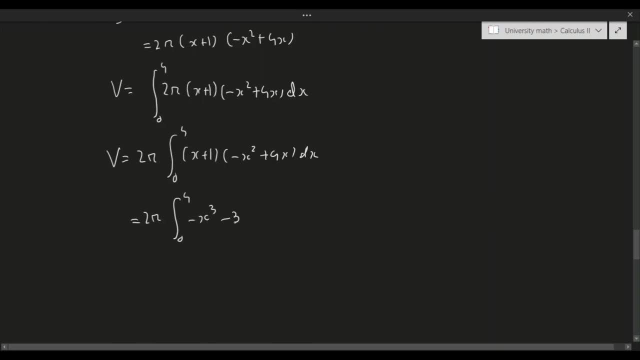 thing. so we get minus x cubed plus 3x squared, plus 4x times dx. so integrating all this, we'll get 2 pi times minus x to the 4, plus x cubed, plus 2x squared from 0 to 4, and that's going to give us 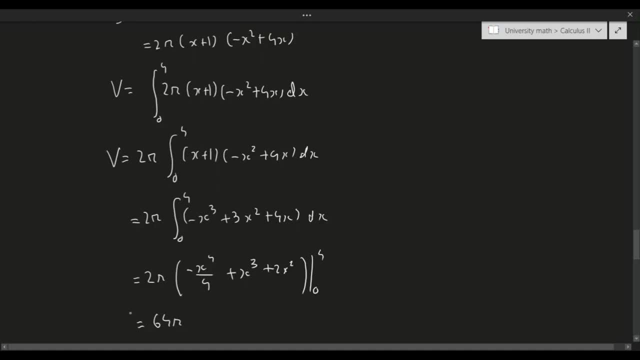 64 pi as our final answer. so that's it for that example. so let's move on to the next example. now let's do the next one. so example okay. so this one is similar. so determine the volume of the solid obtained by rotating the region bounded. 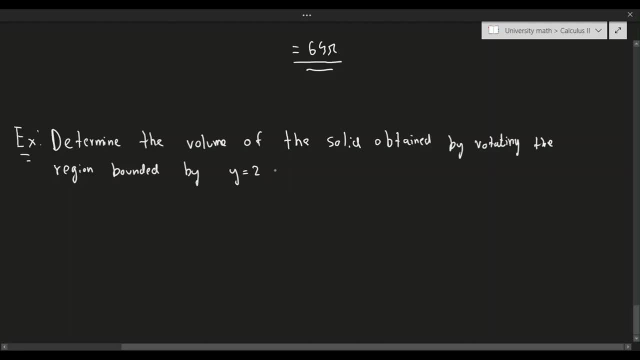 by y equals 2, square root of x minus 1, and y equals x minus 1. about x equals 6. okay, so let's take a look at what's going on here. so let's draw an axis and let's make this over here, actually, as a matter of fact, 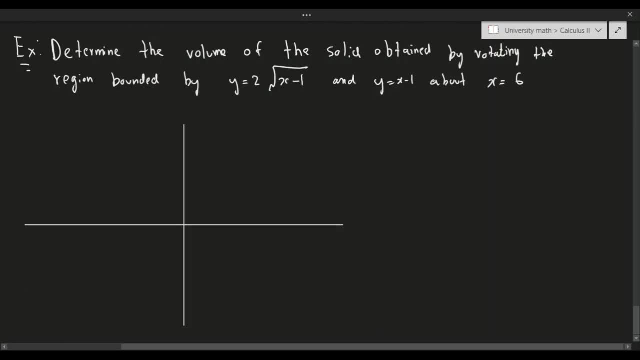 okay, so here is the square root graph, here is the line, and: Okay, so this is the graph. y equals 2 times the square root of x minus 1.. This is the graph. of y equals x minus 1.. This intersection point right. there will be 5.. 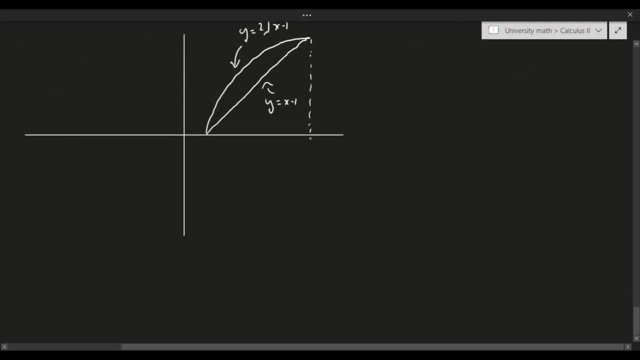 You will figure out how we got to 5 later. So that's 5, that's 1.. And let's go ahead and draw the line of rotation. So that's going to be x equals 6.. So we have to figure out these intersection points. 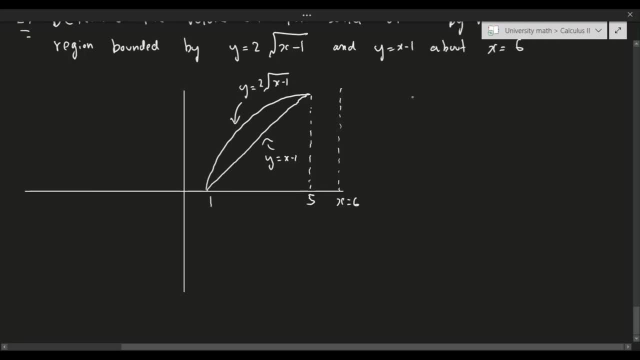 I wrote them down, but let's actually go ahead and actually find them. So once again we set these equal to each other. So 2 times x minus 1 is equal to x minus 1.. So now we square both sides. 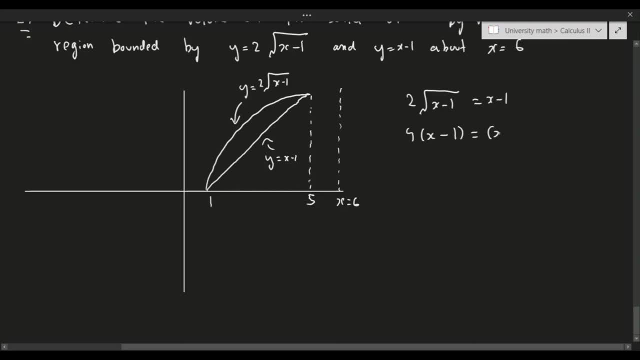 So that's going to give us 4 times x minus 1 is equal to x minus 1 all squared, So that's going to give us 4x minus 4. on this side Over here, we're going to get x squared minus 2x plus 1.. 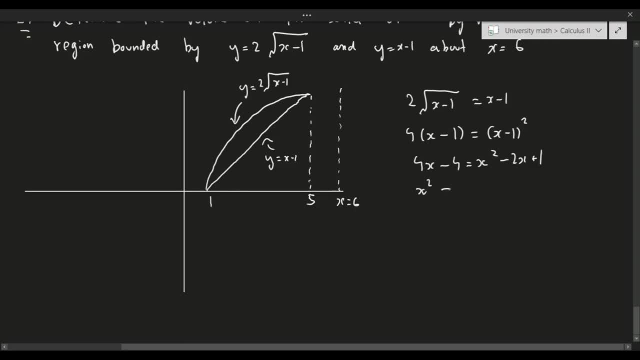 So if I kind of move around, Okay, So if we're moving to one side, we'll get x squared minus 6x plus 5 is equal to 0.. In factoring we'll get x minus 1 times x minus 5 is equal to 0, which implies x equals. 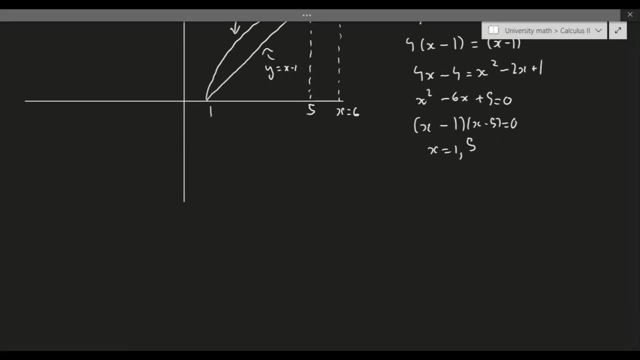 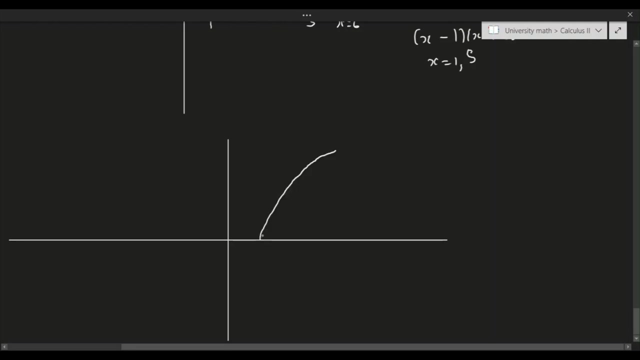 1 and 5.. Okay, So if you go ahead and expand our axis a little bit so we can kind of see this cross section a bit better, it's going to look something like this: So here is the first part, Okay. 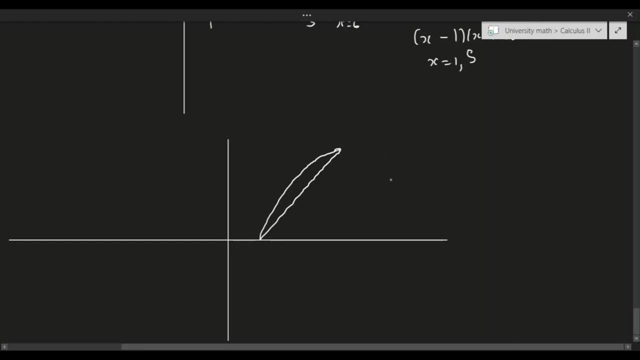 So here is the second kind of part to this, So something like that. Okay, So let's go ahead and draw the cylindrical cross section. So let's draw the axis of rotation, just to be very clear. Okay, So that's going to be 6,, that's 1.. 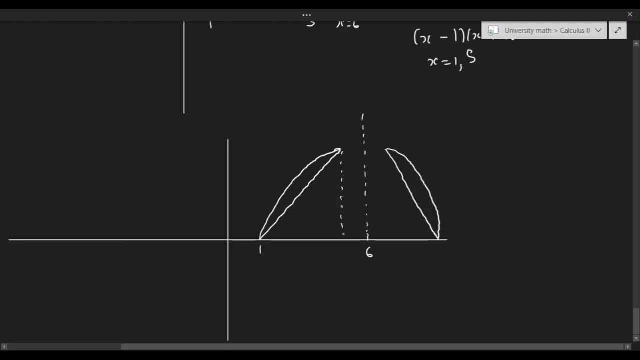 This part right there, that's 5.. And because this is- and let's draw the rest of this- and just to be very clear, that's going to be equal to 11.. We don't necessarily actually need this intersection point, so we're just going to leave it. 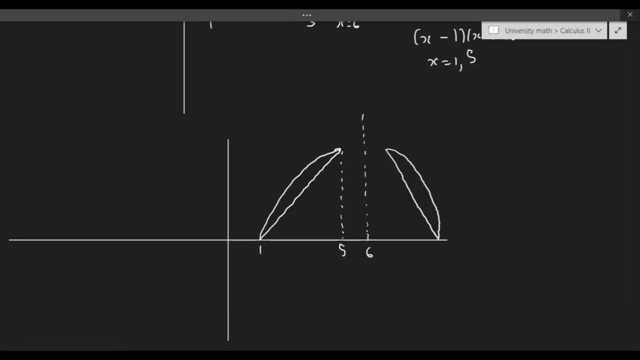 So let's talk about what's going on here. So if I draw the cylindrical cross section, which I'll do using a different color, So it's going to look something like this now. Okay, So here is the cylinder And let's kind of talk about this part. 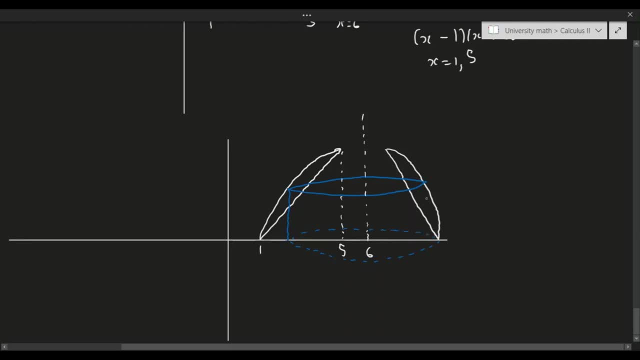 Okay, So here's the other one. Okay, So, in this situation, the height, So height, Okay, Okay, So height is equal to the upper curve minus the lower curve. So, just to be very clear, this curve right there, so this curve, is going to be the difference. 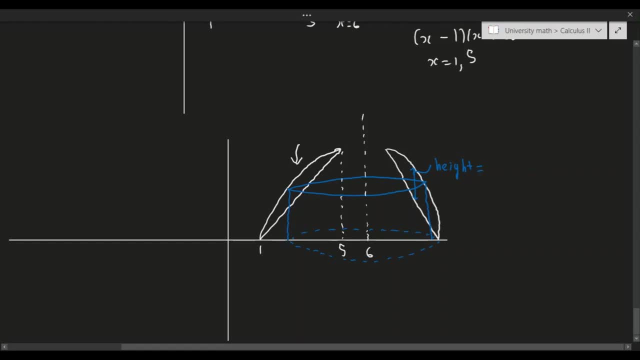 between the higher curve minus the lower curve, So it's going to be 2 root x minus 1 minus x minus 1.. So kind of like that. So in this situation the height is going to be 2 root x minus 1 minus x minus 1.. 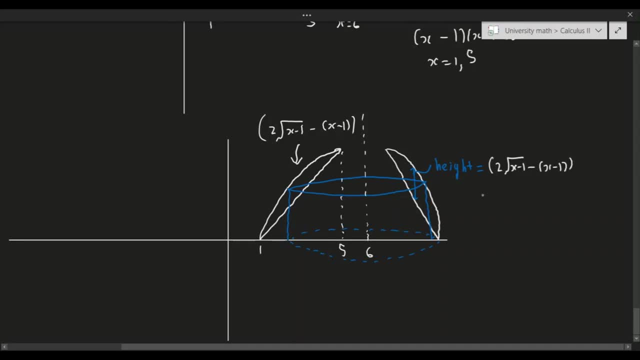 Okay, Okay, So this is going to be 2 root x minus 1 minus x plus 1.. So that's the height And the radius in this situation. so that's going to be whatever this distance is. Okay. So in this situation, the radius is going to be the distance between the end of the 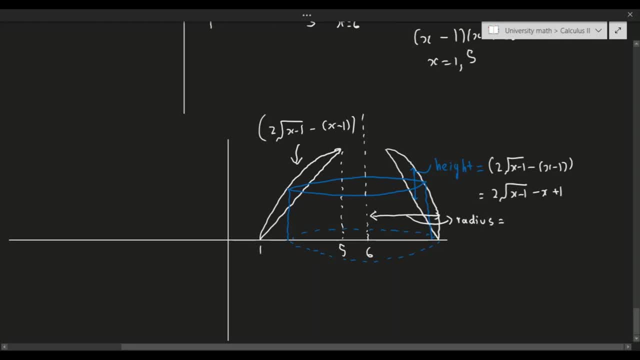 graph to the axis of rotation. Okay, So the radius is just going to be 6 minus x. So technically, if you're saying 6 minus x, we should probably be using this kind of radius. Not that it matters, it's just more or less the same thing. 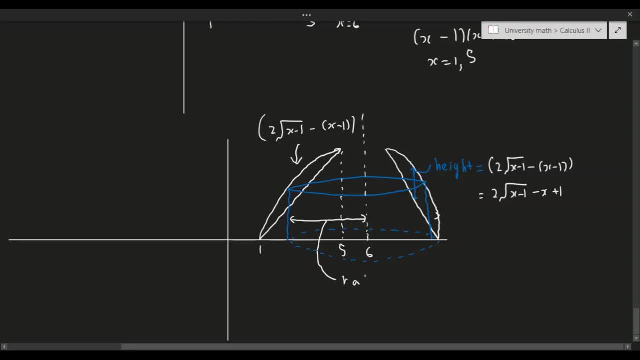 So the radius in this situation is equal to 6 minus x. It's the distance between this line and the end of this graph. Right there, It doesn't matter. We could have used, we could have gone the other direction. It doesn't really matter per se. 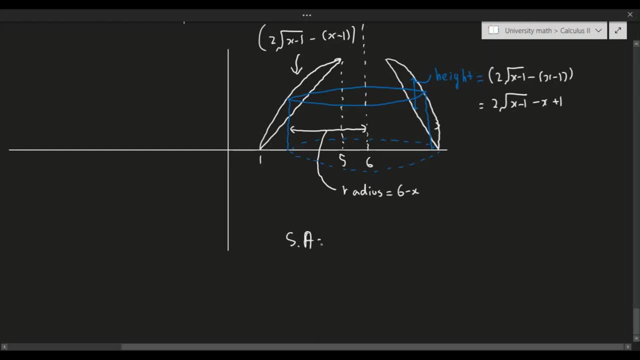 Okay, So in this situation the surface area is equal is going to be equal to 2 pi times the radius times the height, So 2 pi times 6 minus x times the height. So that's going to be 2 square root of x minus 1 minus x plus 1.. 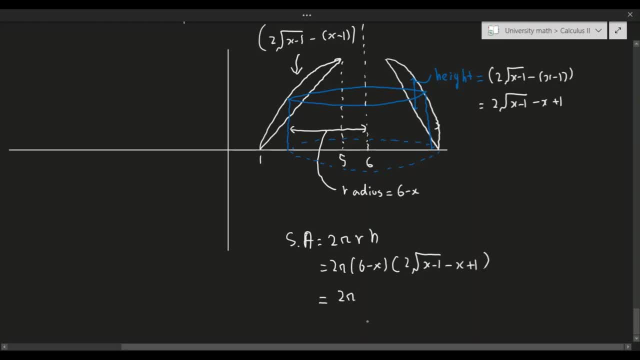 So now we get 2 pi times the integral from 1 to x minus 1.. Okay, So that's going to be 2 pi times the integral from 1 to 5, because that's where we are actually integrating of x squared or not x squared we're going to be, let's just kind of not. 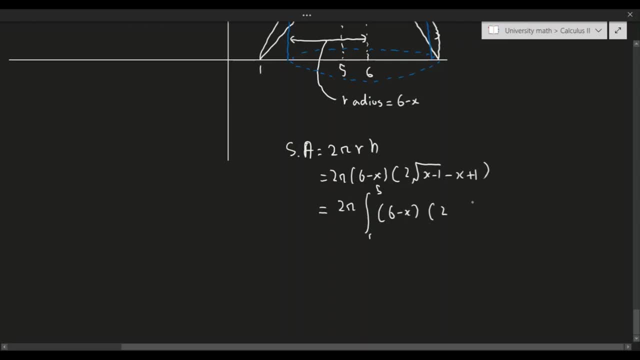 skip steps, So that's going to be 6 minus x times 2 root x minus 1 minus x plus 1 dx, So that's going to be 2 pi times the integral from 1 to 5 of x squared minus 7x plus 6. 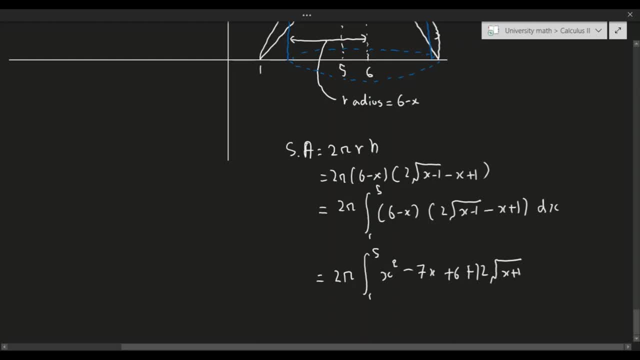 plus 12. square root of x plus 1, or x minus 1 minus 2x. square root of x minus 1 times dx. Now, most of this integral is fairly simple, except this one is a little bit harder to do, So I'm going to do that integral on the side right here.